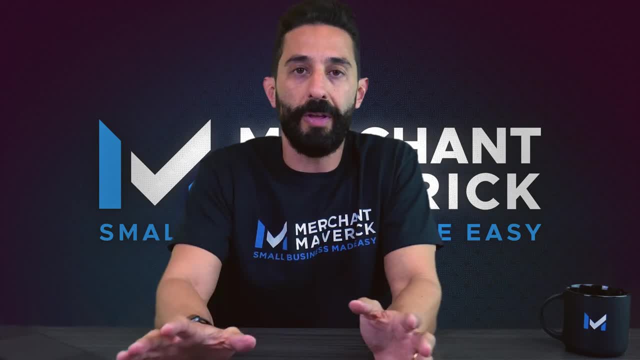 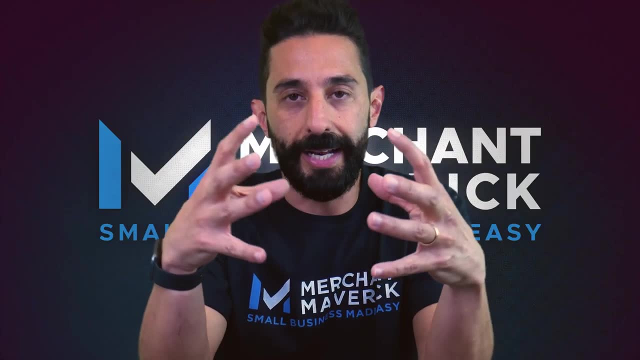 you might want to check out another leading player, Ecwid. They both have a ton of features, very similar features, but there are some key, important differences between the two and we're going to find out what those are. So in today's head-to-head, we're going to compare. 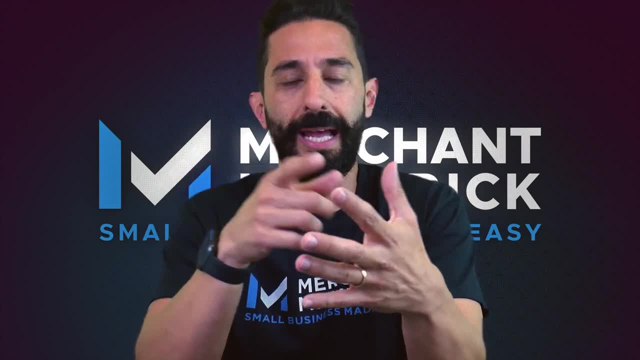 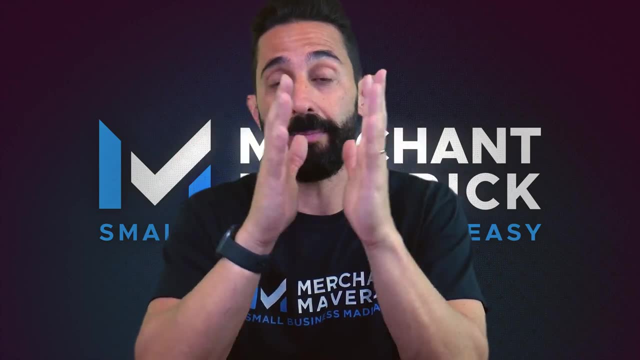 features, pricing, ease of use, customer support and reviews and comparisons and integrations to find out which one of these platforms is better for you. Not necessarily better in general, but better for you. But before we get started, make sure you click that subscribe button. 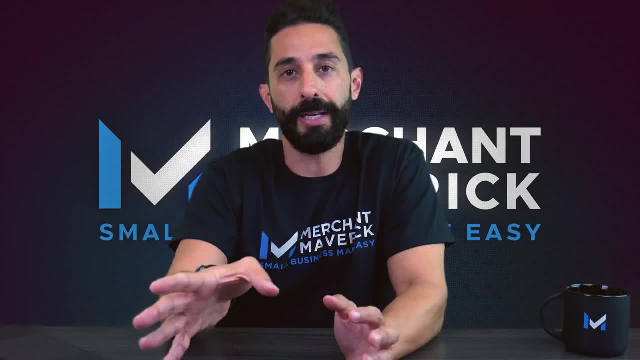 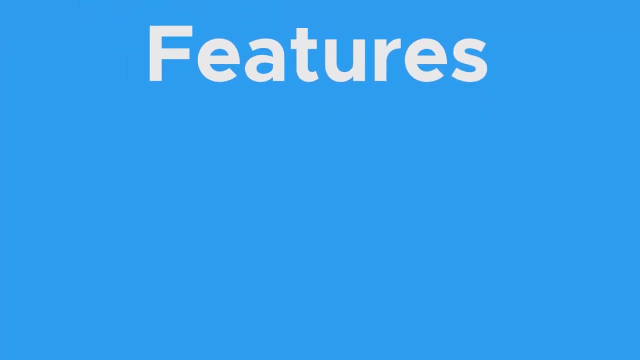 hit the alert bell so you can be notified every time we publish new content here at Merchant Maverick. All right, so let's get started with features, both of which are very similar, but there are some key differences between the two. Both of them, out of the box, have very basic, good features to help you get started with selling. 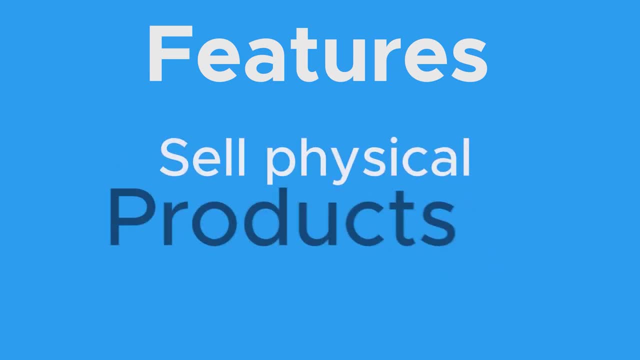 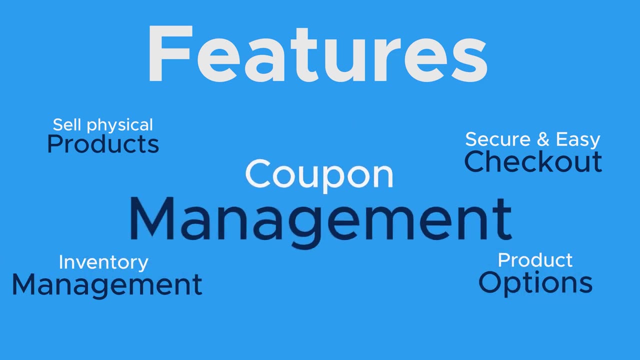 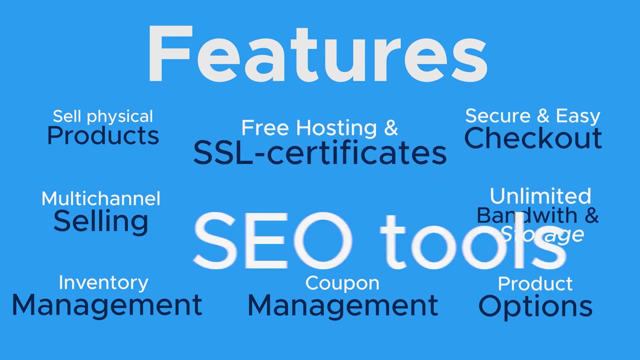 online. Some of those basic features are going to include the ability to sell physical products, secure and easy checkout, inventory management, product options, coupon management, multi-channel selling, unlimited bandwidth, unlimited storage, free hosting and SSL certificates, SEO tools and more. Again, pretty much everything that you need to sell online. 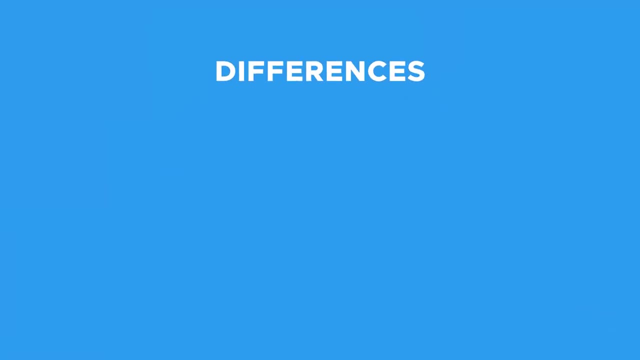 but let's look at what those key differences are. First off, if you're trying to sell digital products like digital eBooks or whatever information products, you're going to have that feature built in with Ecwid but not with Shopify. With Shopify, you're going to have to add a third. 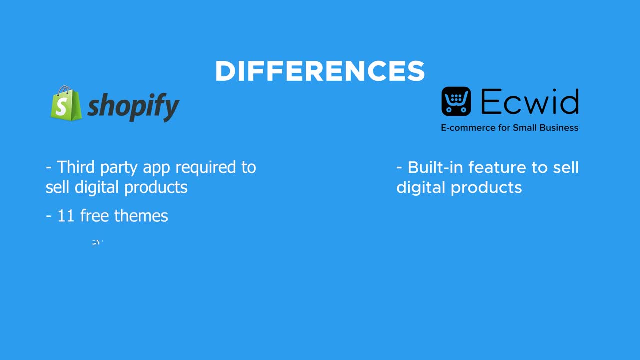 party app in order to sell digital products. When it comes to free themes, Shopify is the winner here. They offer 11 beautifully designed free themes, whereas Ecwid offers a whopping one. If you're a blogger, a writer, you want to add blogging functionality to your eCommerce platform. 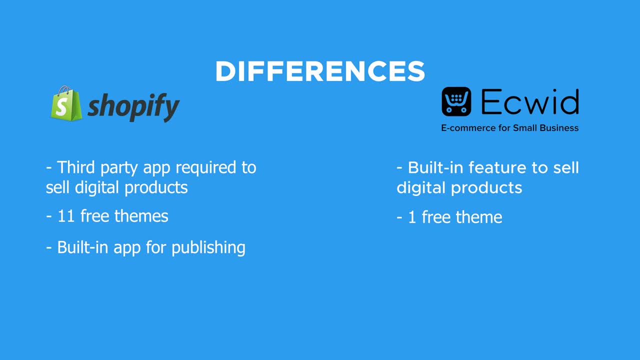 you want to publish content, then you're going to have that built-in built-in functionality with Shopify's platform, but you're not going to have it with Ecwid. If you're a drop shipper and you want to drop ship, Shopify has a direct integration with one. 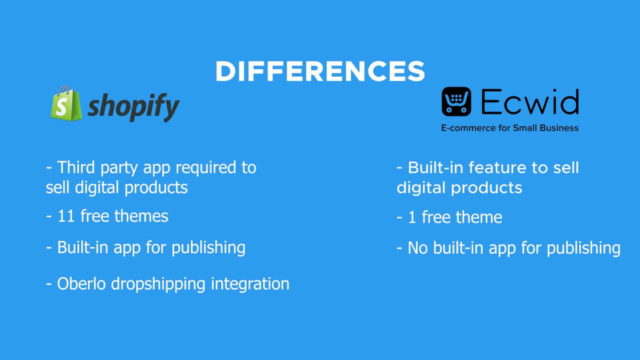 of the biggest drop shipping platforms, Oberlo. With Ecwid, on the other hand, you're going to have to install a third party app. And, lastly, if you need fulfillment services, Shopify offers in-house fulfillment, whereas with Ecwid, you're going to have to use a third party. 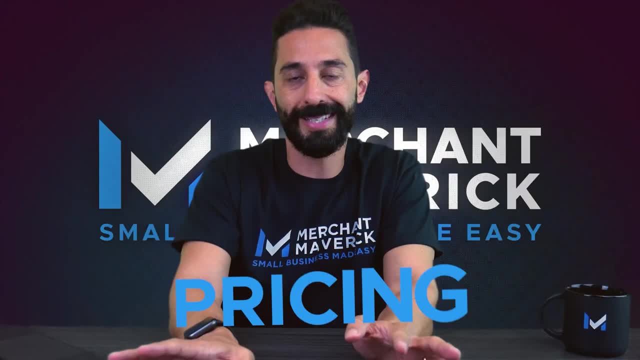 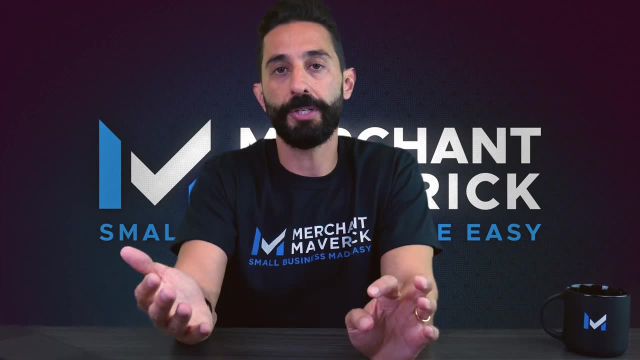 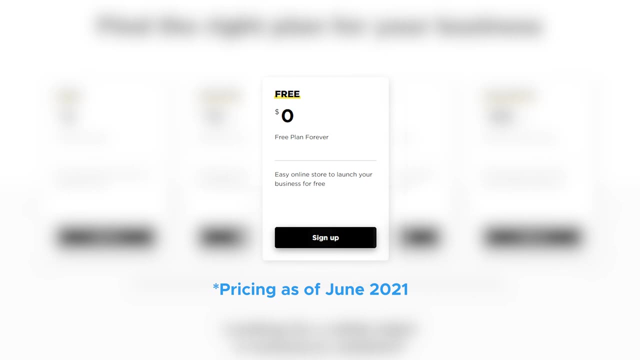 like RedStag or ShippyPro. All right, let's move on to pricing. Ecwid has four very simple, straightforward pricing plans, and they all increase in price and functionality as you move up. Starting with the free plan, which is surprisingly $0 a month, offers you the ability to sell up to 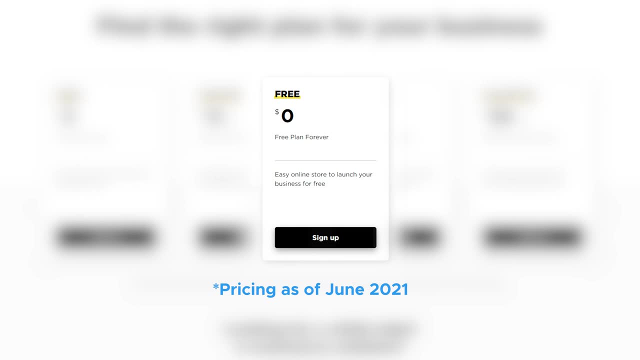 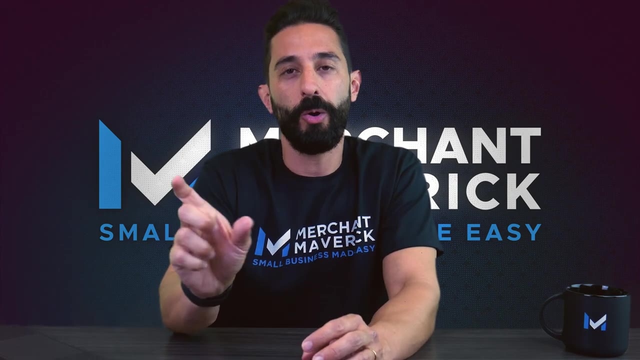 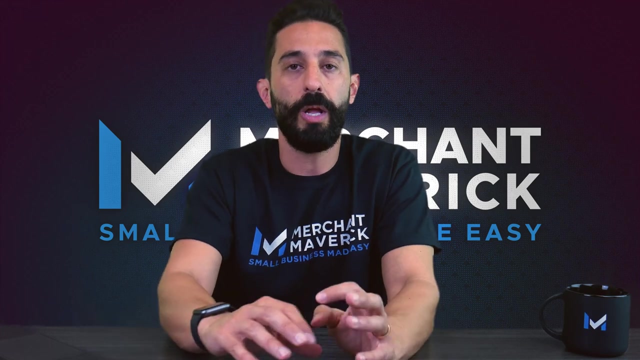 10 products on a one-page website with a built-in online store. The free plan also allows you the ability to sell on multiple social media sites with buy now buttons or social media integrations. the ability to sell in person in a brick and mortar store with three different point of. 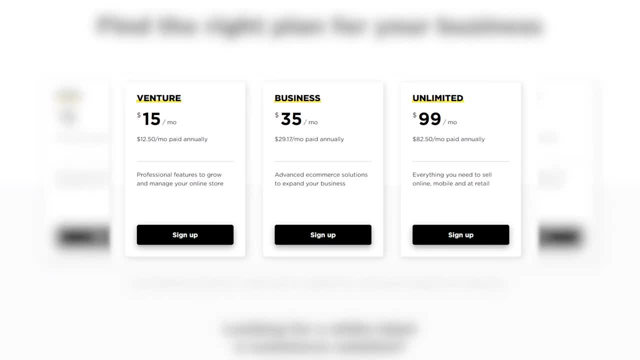 sale integrations. Additional plans include venture at $15 a month, business at $35 a month and unlimited at $99 a month And, as the name implies, unlimited allows you to list as many products as you like and you can add any number of staff accounts under the unlimited plan. Moving on to Shopify's pricing, Ecwid compares a little bit more favorably here, as they offer a free plan, whereas Shopify does not. Shopify's lowest plan is Shopify Lite at $9 a month, which is very similar to Ecwid's free plan. Shopify's most popular plans are basic. 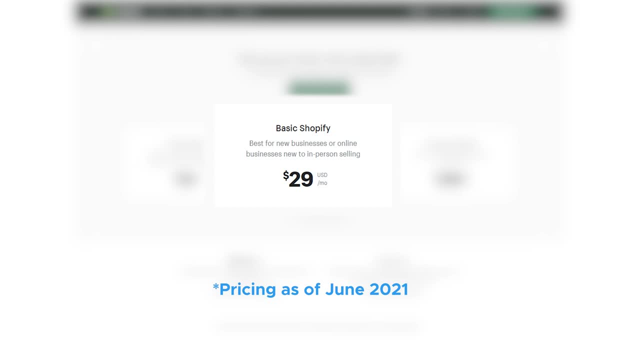 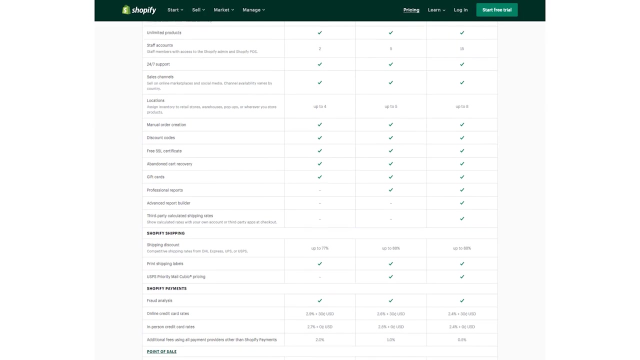 Shopify at $29 a month plus a 2% per transaction fee, regular Shopify at $79 a month plus a 1% per transaction fee or Shopify Advanced at $299 a month plus a half a percent per transaction. Under the basic Shopify plan you can set up a standalone e-commerce site, a blog you can add. 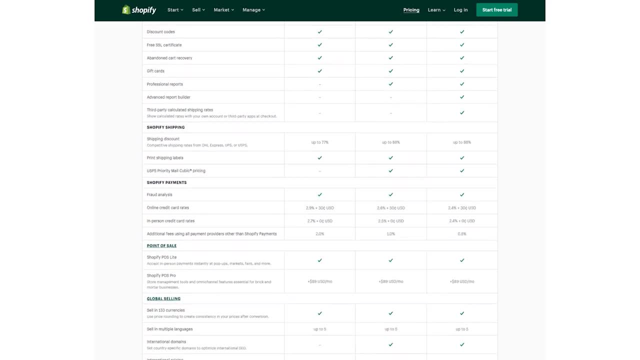 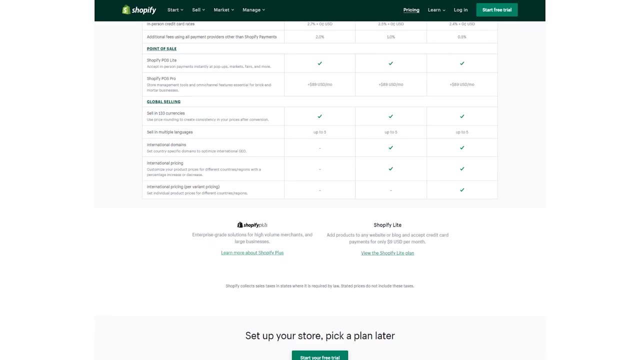 unlimited products and add two staff accounts. Each plan offers more functionality and features, with the Advanced plan allowing up to 15 staff accounts and up to eight locations. You'll notice that there's a per transaction fee added to the monthly cost of every Shopify plan. which genuinely sucks, But you can get that transaction fee waived if you use Shopify's in-house app. You can also add a monthly fee to the monthly cost of every Shopify plan- which genuinely sucks, But you can get that transaction fee waived if you use Shopify's in-house app. 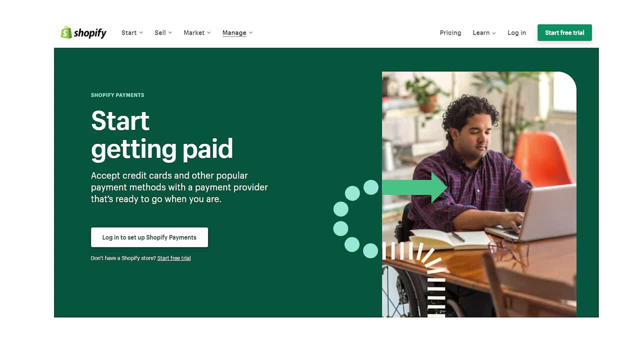 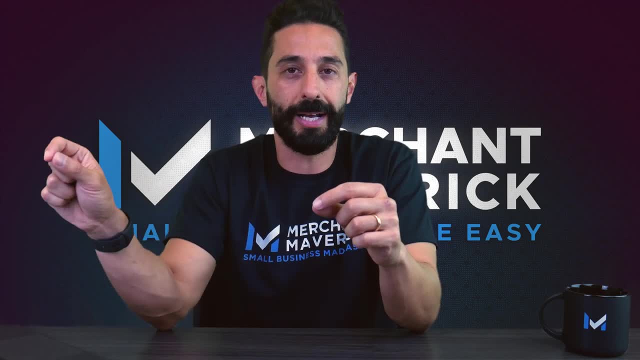 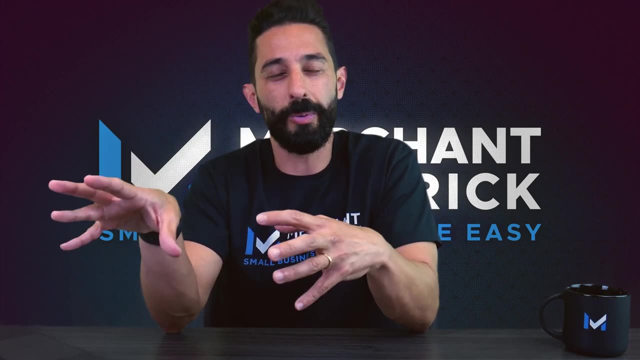 Payment processing service called Shopify Payments that'll give you the ability to accept credit cards directly through Shopify, waiving that additional pointless transaction fee that you'll have to pay. You'll just end up having to pay credit card processing fees, which generally run from 2.4% to about 2.9%, depending on the type of transaction. 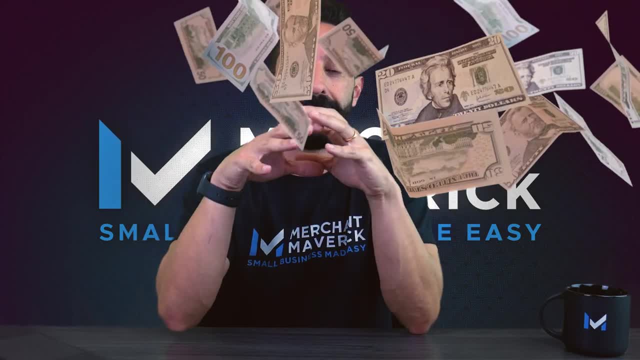 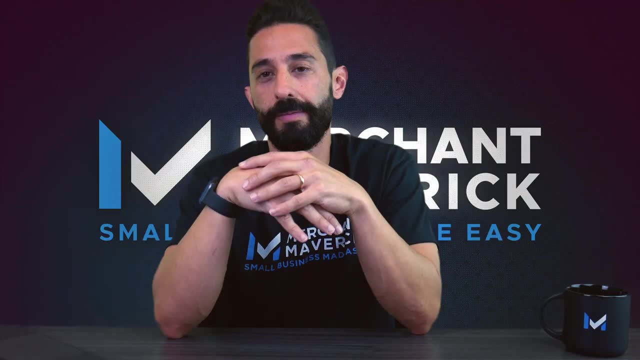 And if you're a big e-commerce platform, you're a big dog, you're selling thousands and thousands of products, you're doing millions and millions of dollars in revenue and you need some white glove service or you need additional help, then you can do Shopify Plus, which is their enterprise platform. 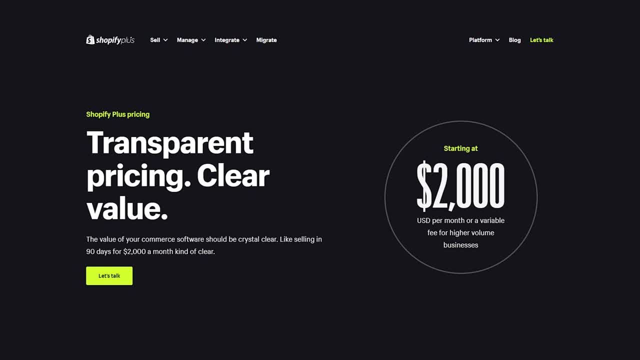 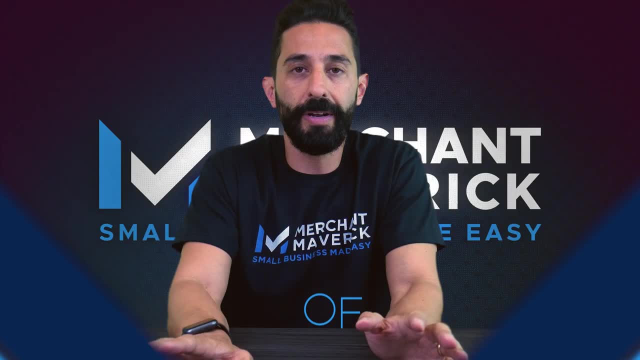 It's very much a customized solution. You'll probably have to talk to a Shopify rep to even get pricing, but really it's like the next level of service beyond the regular plans. Moving on to ease of use, both platforms are very easy to use without any overly complicated. 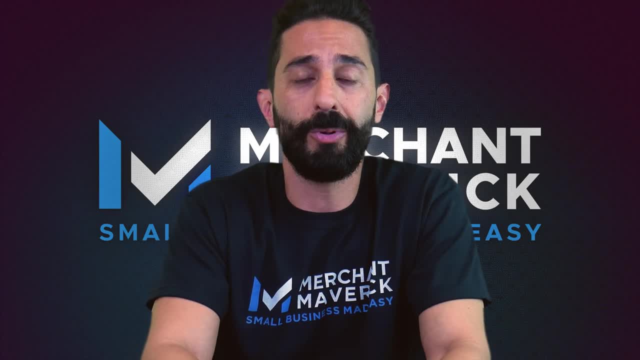 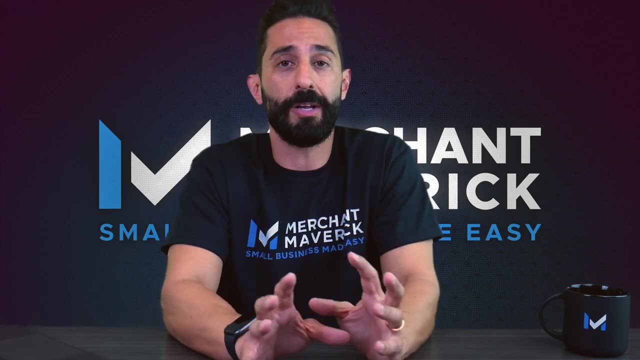 processes, making them perfect for those of you that want a simple, easy user interface. But all that simplicity comes with a price. If you want a simple platform, you're going to have to sacrifice on the functionality side, which means that you're 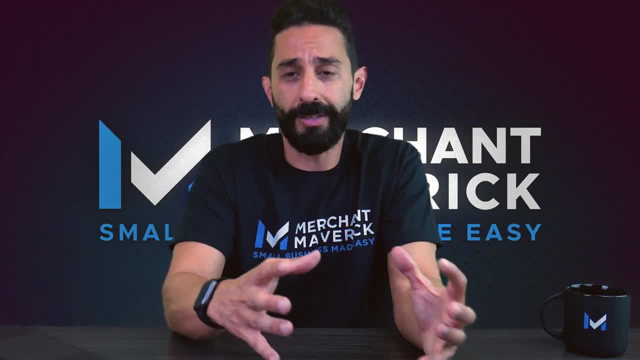 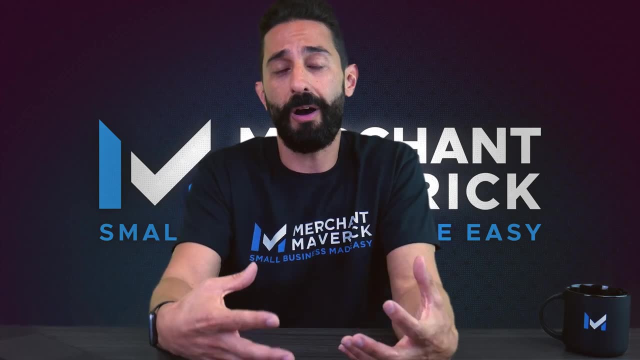 going to have to engage in adding add-ons and apps and integrations, And those apps are sometimes owned by third parties that charge an additional fee, So the cost can balloon if you really want to add functionality to your e-commerce platform. So, to summarize: ease of use. they're both very 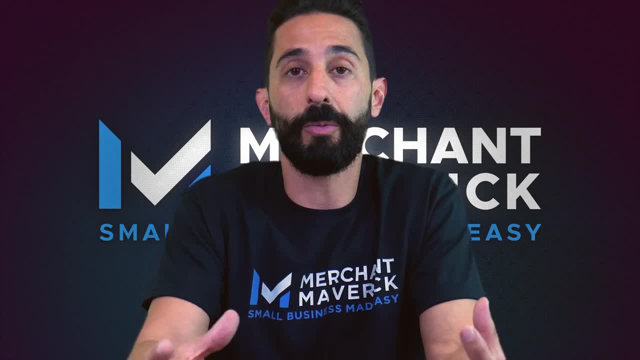 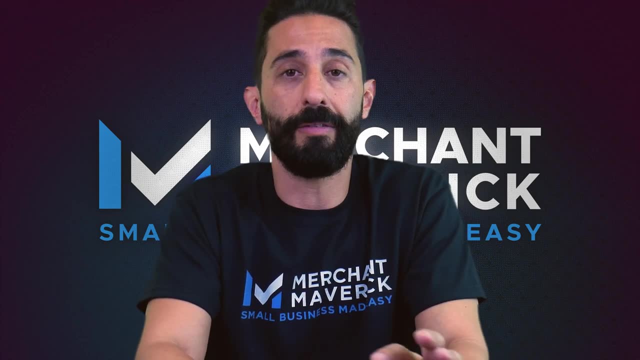 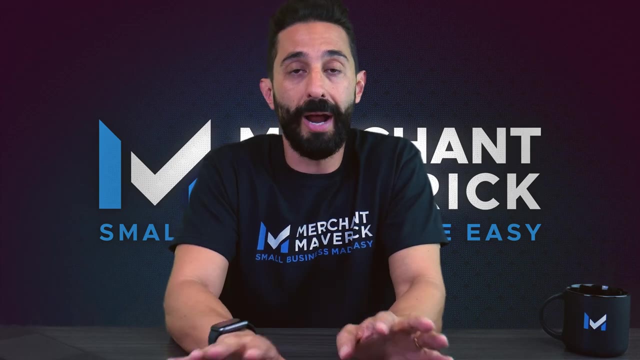 easy to use. They're both limited in functionality. They both kind of rely on third-party apps, but Ecwid has a little bit more functionality in-house. But again, both of them are very easy to use. Moving on to customer service and support, both Shopify and Ecwid offer support in a variety of 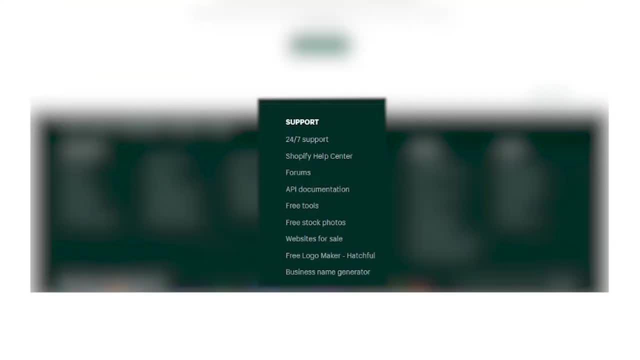 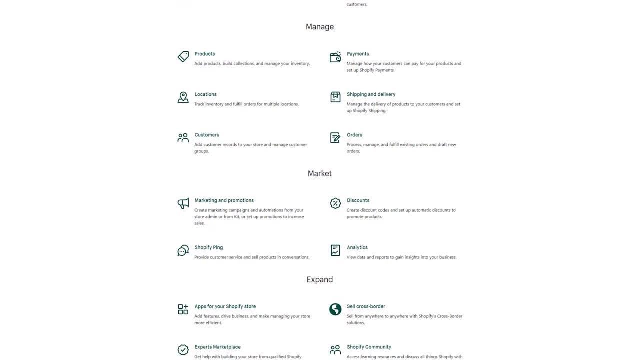 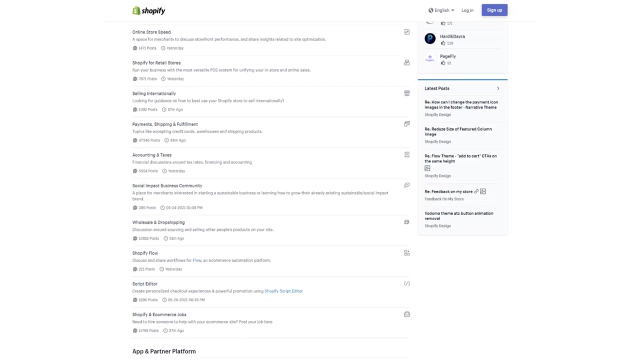 ways. Shopify provides phone and email support, live chat, forums, a help center, webinars, a blog and other free tools for making the most of the platform. Shopify also offers full API documentation and other resources for those who are technically inclined, and also maintains a 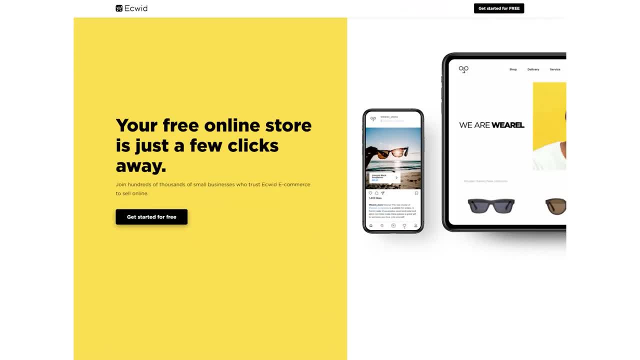 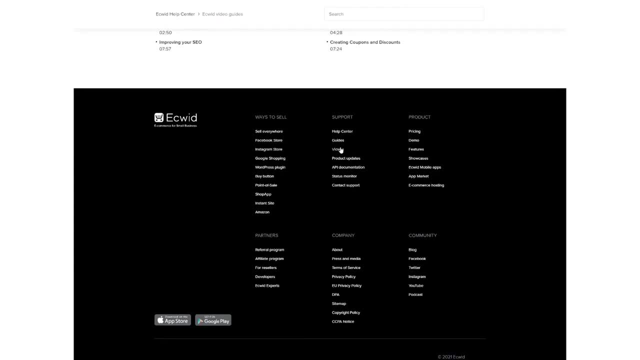 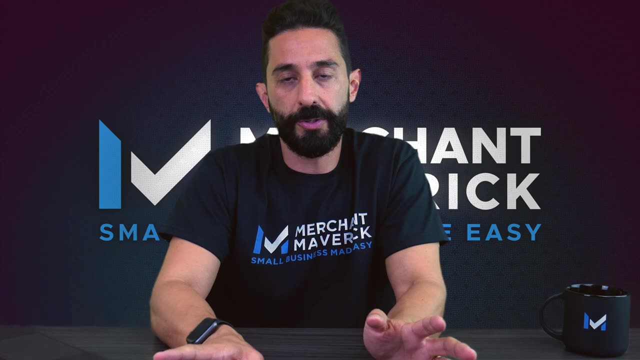 mobile phone. To help you keep your phone safe and secure, Shopify offers a number of support options. It's also available on the Google Play Store and YouTube channel. Ecwid's support options include email, live chat, a help center, community forum, guides, videos. 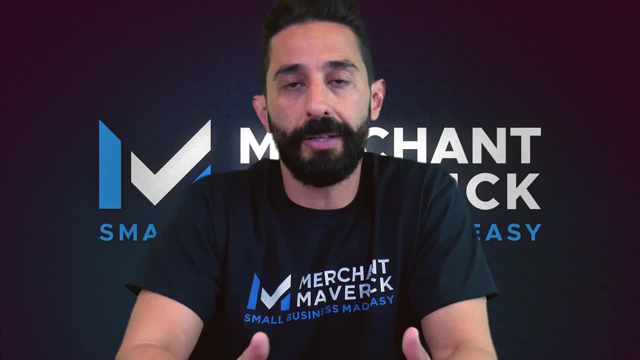 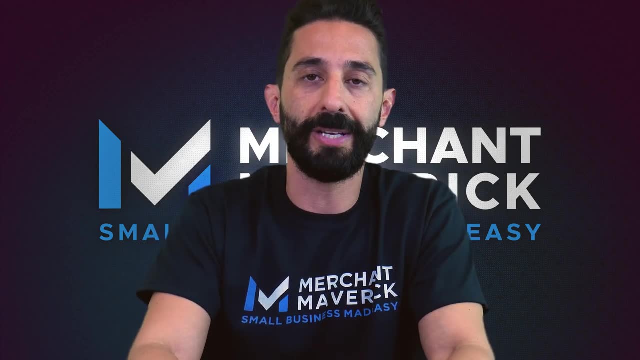 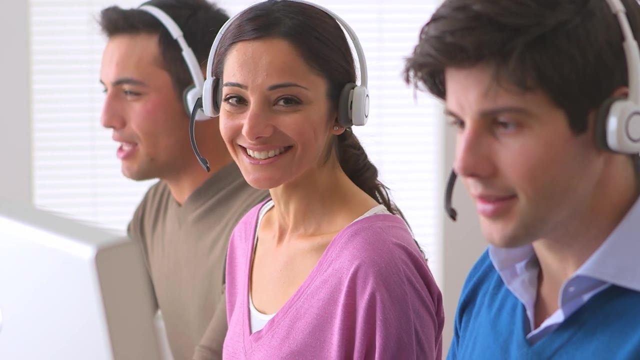 and more. Ecwid users on paid plans can access telephone support too, and users on the top tier can use if you're unable to get that full service from ecwid. shopify support garners mixed reviews too. some users are happy with the helpful, friendly support that they receive from shopify. 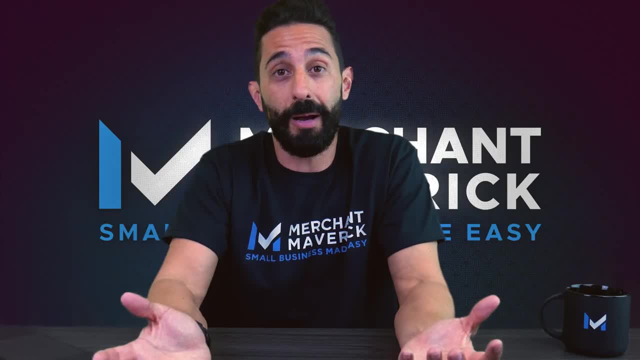 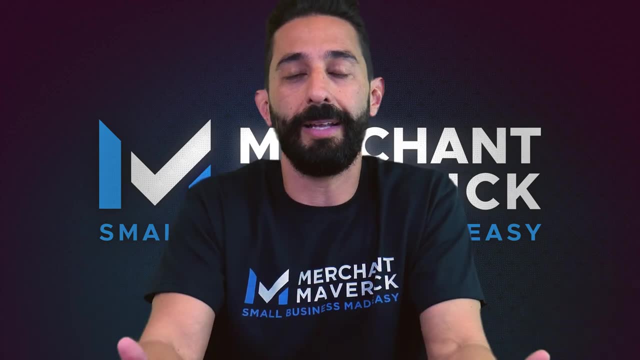 representatives and others sometimes receive the exact opposite. it's kind of a crapshoot depending on which representative that you get, but i guess that's the same for a lot of big companies. again, if your representative isn't so helpful, you have so many self-help options that if you just do a 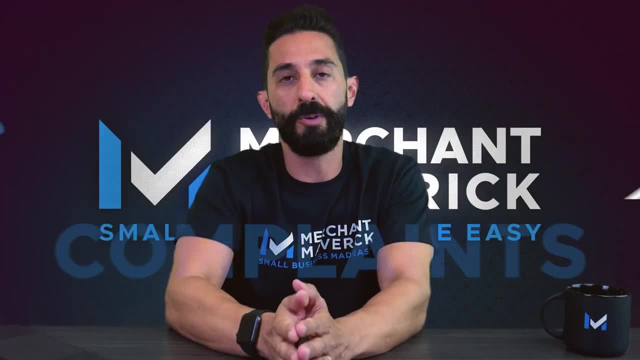 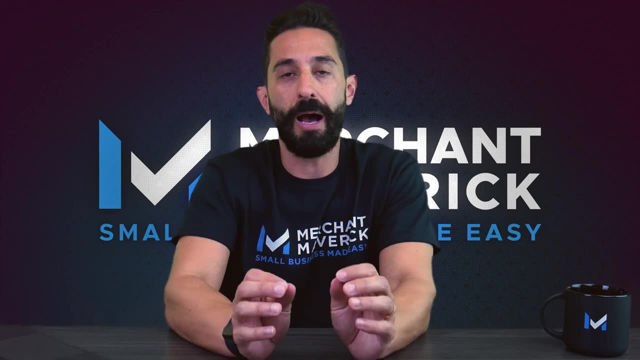 little bit of digging, you probably find the answer yourself. all right, let's move on to reviews and complaints. both platforms receive more praise than they do complaints, but let's cover some of those complaints, however small they are. as i mentioned before, some ecwid users are definitely upset. 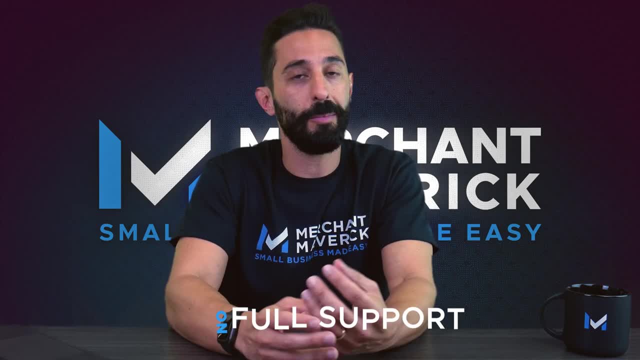 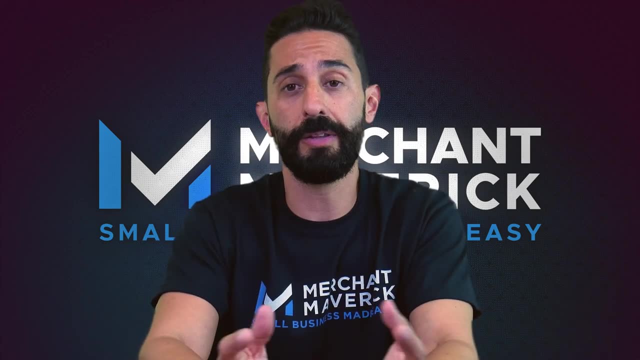 about the fact that they don't get full support on the lower level plans. but again, it's to be expected. it's a free plan. you can't get that much cheaper than free. another complaint is that there are limited features on the free plan. it's a free plan. what can i say? it's a free plan. 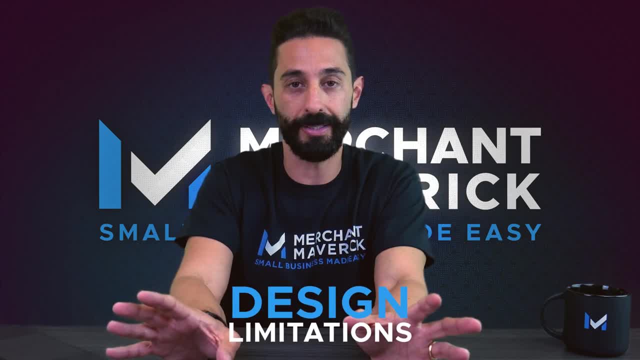 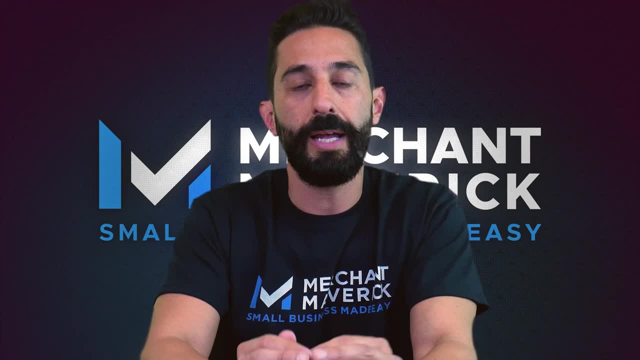 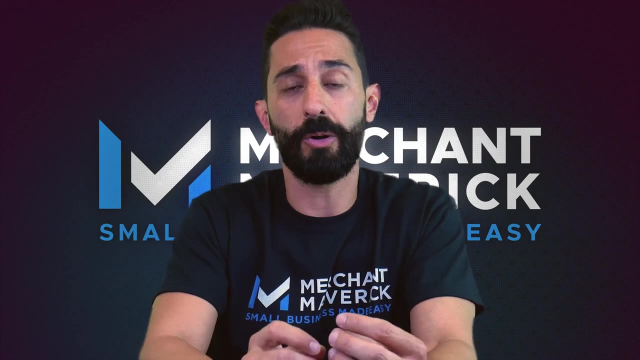 and the last complaint is that there are design limitations, and this one makes sense. there's only one free theme that you can use really, and that's it. on the flip side, ecwid users praise the simplicity, the ease of use, the low cost, the ability to integrate across multiple social 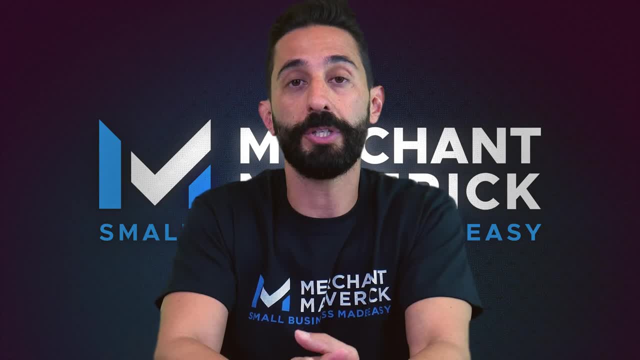 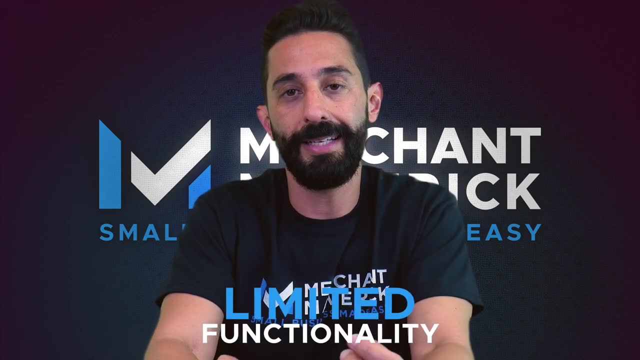 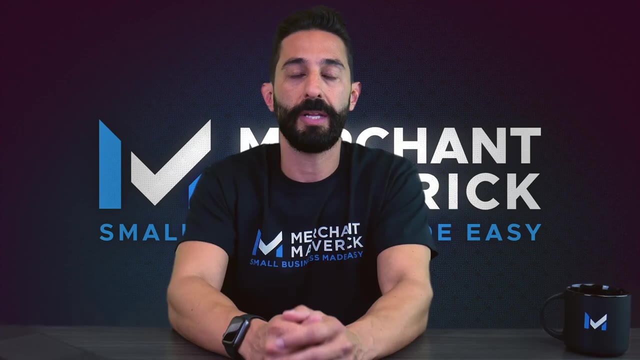 media channels and also the multilingual functionality, the ability to sell in multiple languages. as for shopify, the most common complaints are limited functionality and the necessity to purchase add-ons to increase that functionality, which obviously becomes costly for some. and of course, nobody likes to pay the transaction fees. the transaction fees can be waived. 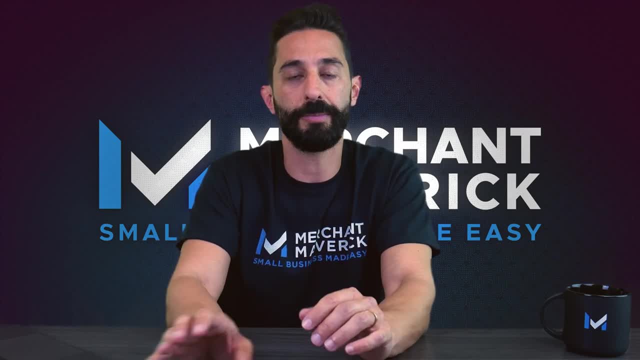 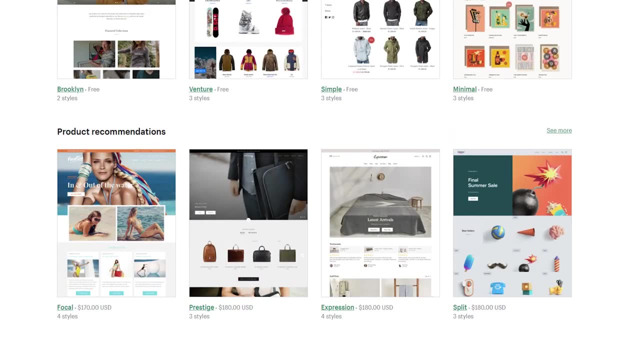 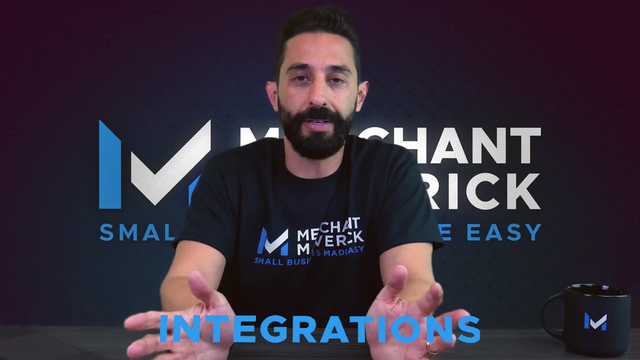 though, if you use shopify payments, their in-house payment processor. shopify users praise the platform's ease of use, multiple beautiful themes and the abundance of integrations that allow you to customize your e-commerce experience. speaking of integrations, this is one area where shopify is a clear winner. up until now, in the different areas, they've kind 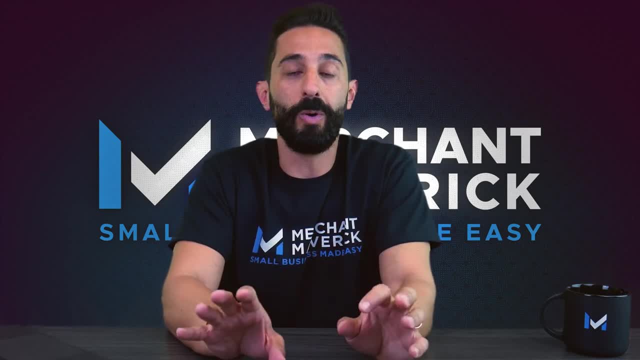 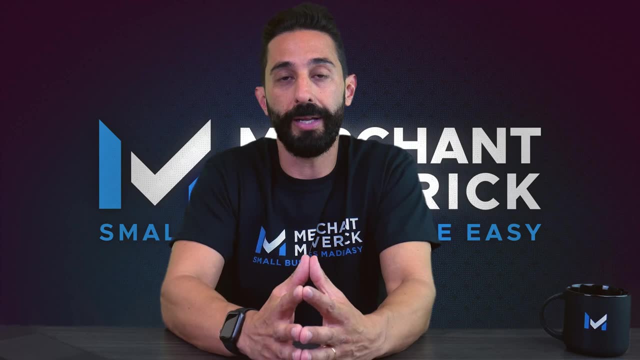 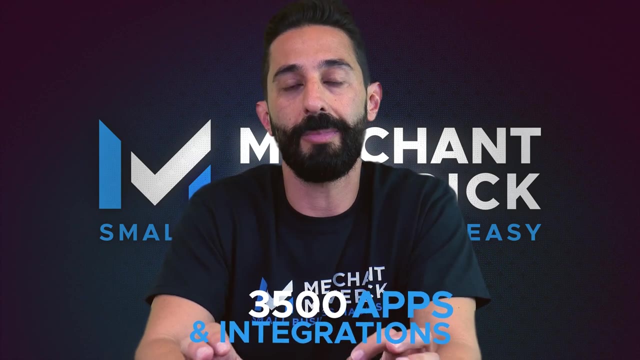 of been head to head, but when it comes to integrations, ecwid has a smaller number of integrations that you can only access when you're on premium plans and not the free plan, whereas shopify offers over 3 500 apps and integrations that can help you customize your store in really. 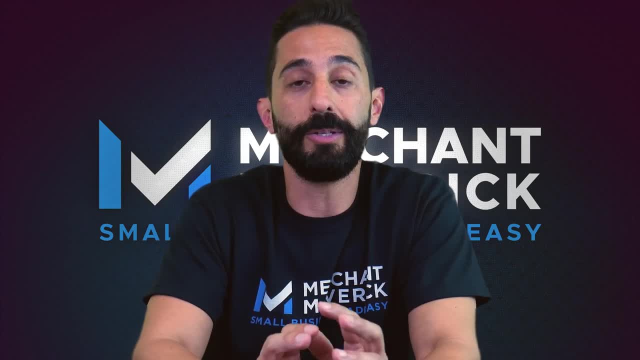 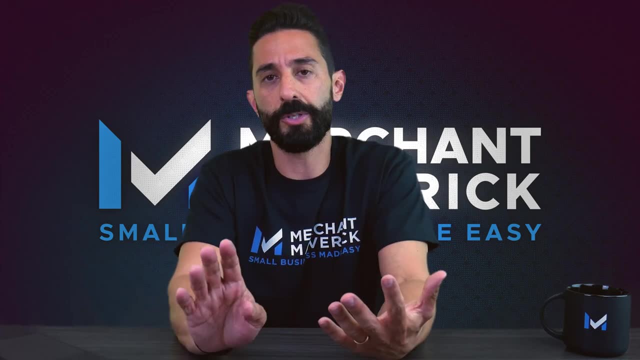 any way that you would like, and in ways that you probably don't even know, that you could increase the customization. so, now that we've covered features, ease of use, integrations, customer support, reviews and complaints, which one of these platforms is right for you you're going to want to choose?